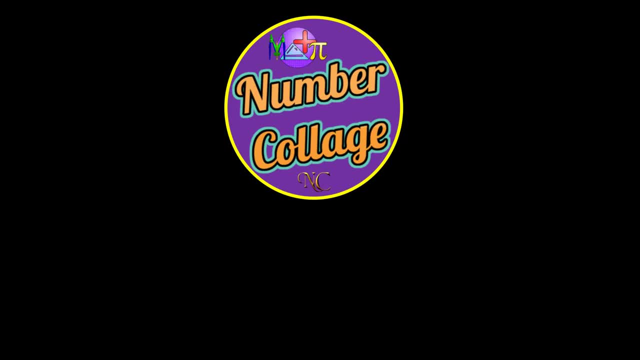 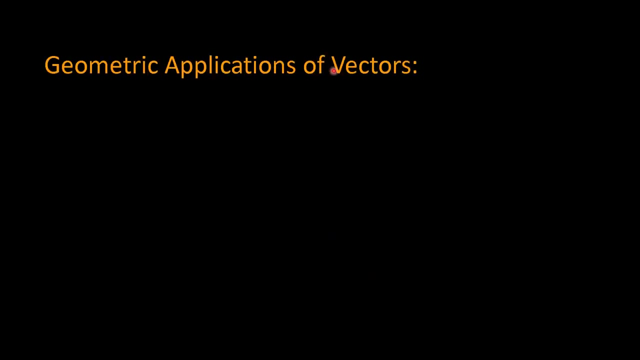 Hello friends, you are watching channel number collage. This is my sincere effort to help you understand basic mathematics in a simple and easy manner. In this video we will discuss geometric applications of vectors in which we will prove important results, properties, theorems and geometry by using vector method. We will write position vectors of various 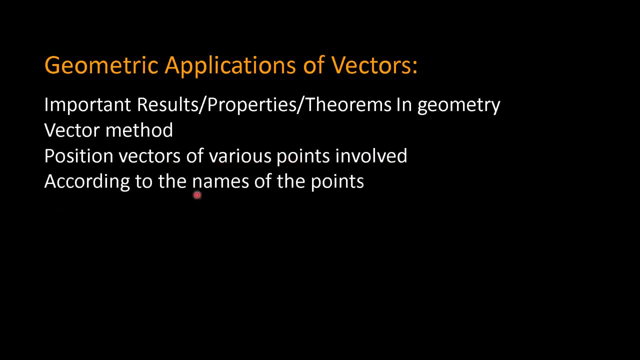 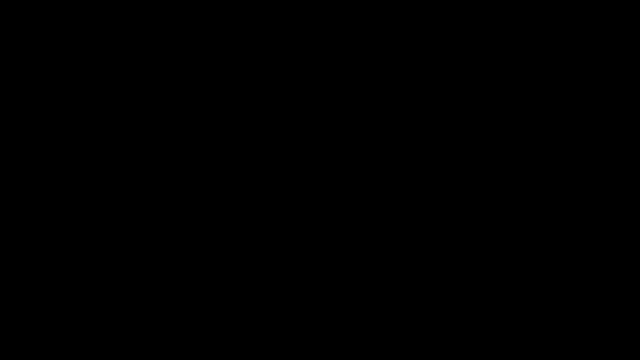 points involved according to the names of the points, without any special mention. For example, we will write position vector of point A as A bar, that of point R as R bar and that of G as G bar, so and so forth. Result 1 is in two parts. The first part is radians of a triangle are concurrent In triangle. 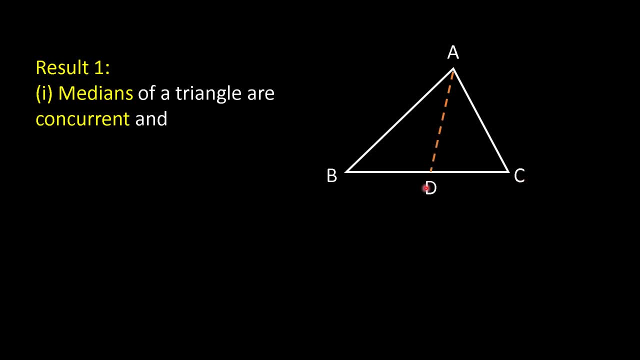 ABC, radian AD is non-concurrent. Radian AD, radian BE and radian CF are concurrent, which means they pass through the same point. The second part is the point of concurrency, which is this point divides each radian in. 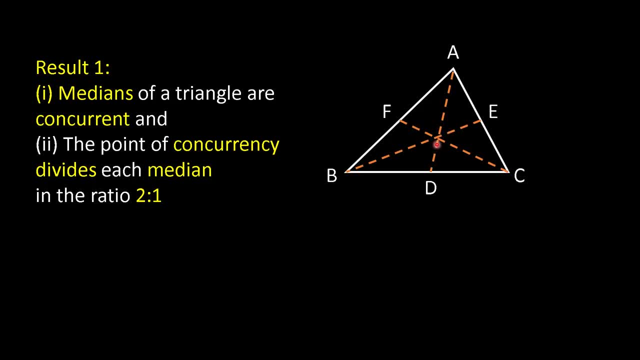 the ratio 2 as to 1.. So this point divides radian AD, radian BE and radian CF in the ratio 2 as to 1.. The third part is the point of concurrency, which is- this point is known as centroid. 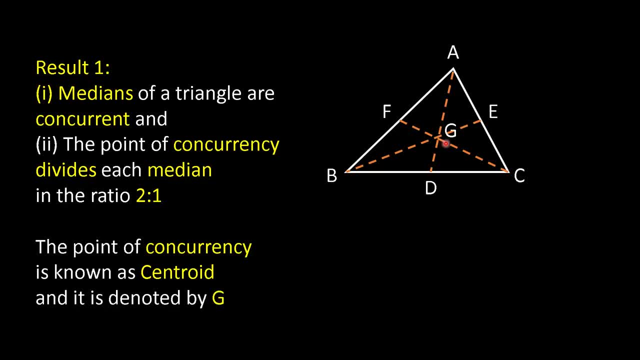 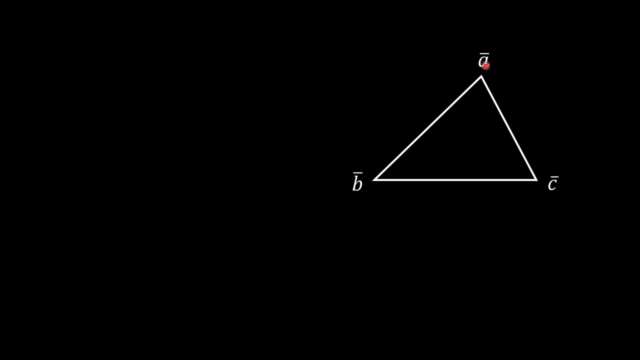 and it is denoted byiful kiG. We have to prove that G divides each of the radians in the ratio 2 as to 1.. Result 2: Result 2: Have some минут. Result 3: ывайтесь B of the vertices a bar B, bar C, bar for median ad by midpoint formula. we write: 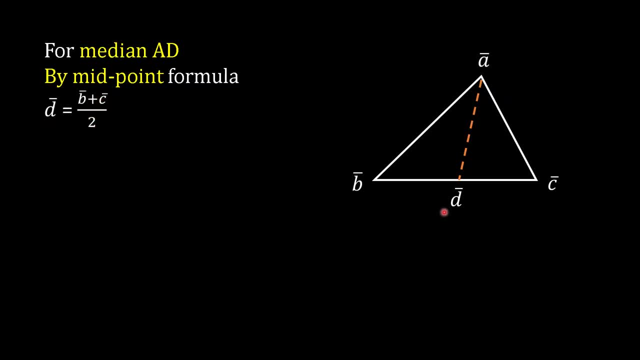 D bar equals B bar plus C bar by 2, so that will be 2 D bar equals B bar plus C bar. there is a bar lacking on the right hand side, so we will add a bar on both the sides and write 2 D bar plus a bar. 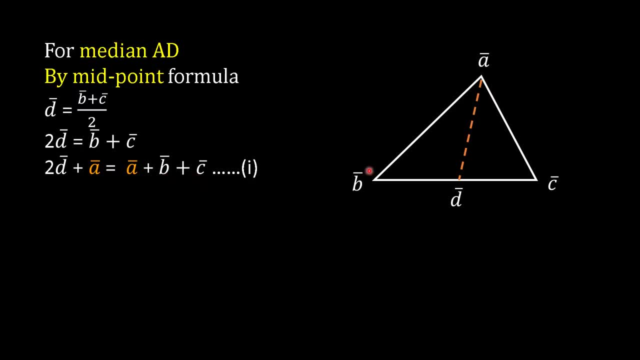 equals a bar plus B bar plus C bar. we name this equation one on the same lines. for median be, we write: 2 e bar plus B bar equals a bar plus B bar. equals C bar. equals D bar. equals C bar. equals D bar plus C bar. for median CF, we write: 2 F bar plus C bar equals a bar plus B bar. 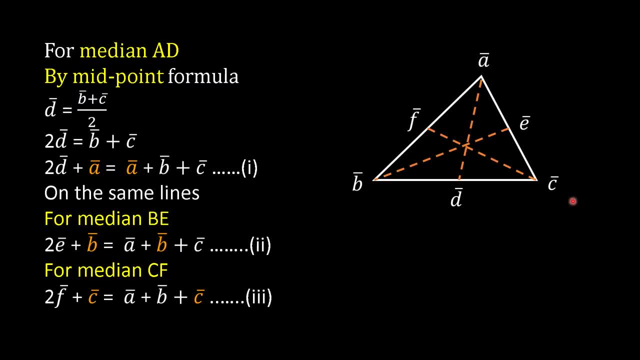 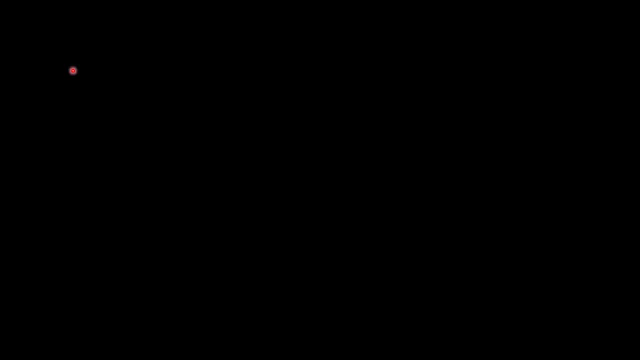 plus C bar. we name this equation 3. we will rewrite these three equations. we will rewrite these three equations. we will rewrite these three equations. equation 1, 2, 3: we observe that the right. equation 1, 2, 3: we observe that the right. 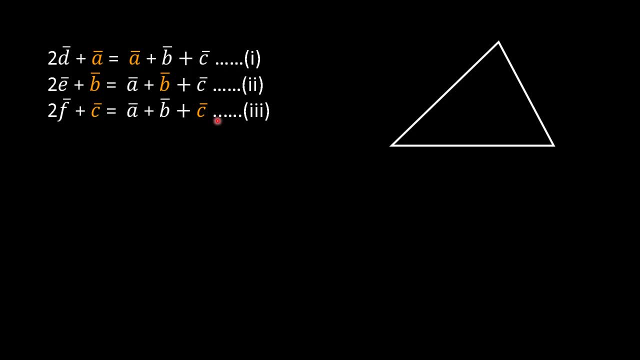 equation 1, 2, 3. we observe that the right side of these three equations is same side of these three equations is same side of these three equations is same. therefore, their left sides will also be. therefore, their left sides will also be. therefore, their left sides will also be equal. we will divide each of these. 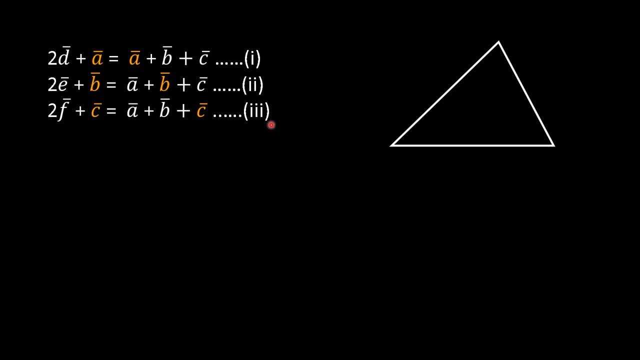 equal. we will divide each of these equal. we will divide each of these equations by 3 throughout and write 2 D equations by 3 throughout and write 2 D equations by 3 throughout and write 2 D bar plus a. bar by 3 equals 2 e bar plus B. 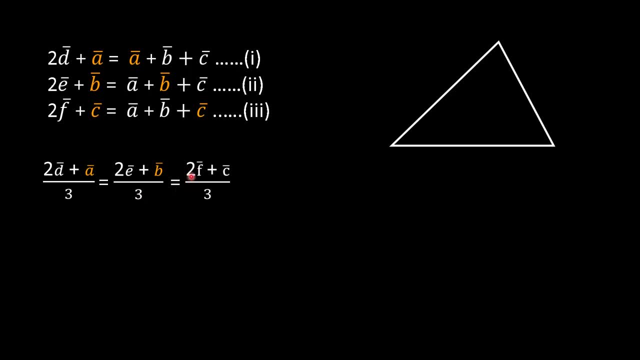 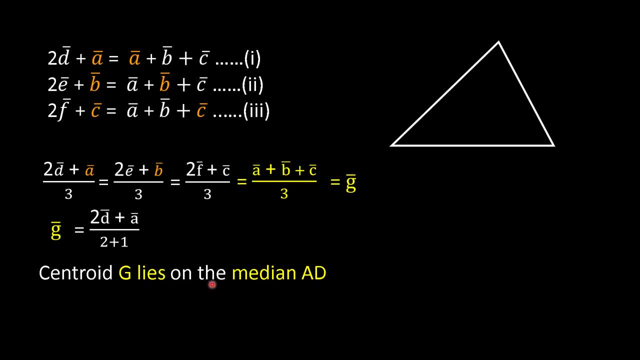 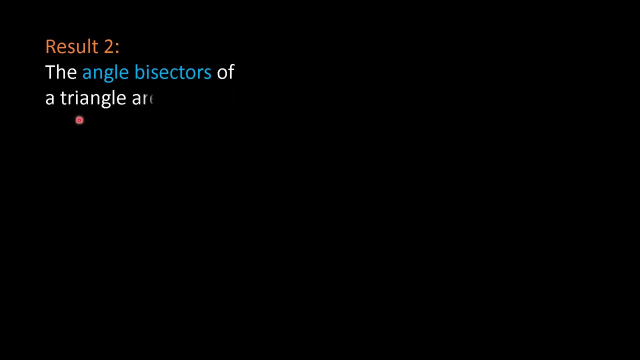 centroid G lies on the median AD and G divides median AD in the ratio 2 as to 1. same can be said about median B, E and C, F. hence that proves result 1. in result 2 we have to prove that the angle bisectors of a triangle are concurrent, which means they pass through the same. 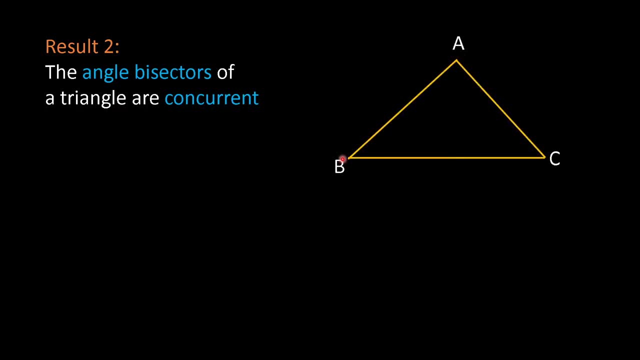 point. so we have here triangle ABC, angle bisector AD, angle bisector BE and angle bisector CF are concurrent, which means they pass through the same point. this is the point. the point of concurrency is known as in center and it is denoted by capital I. so 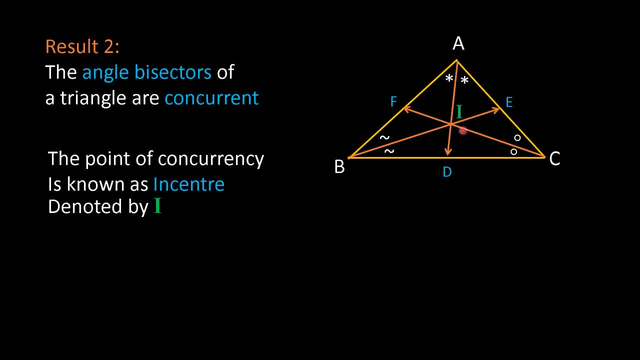 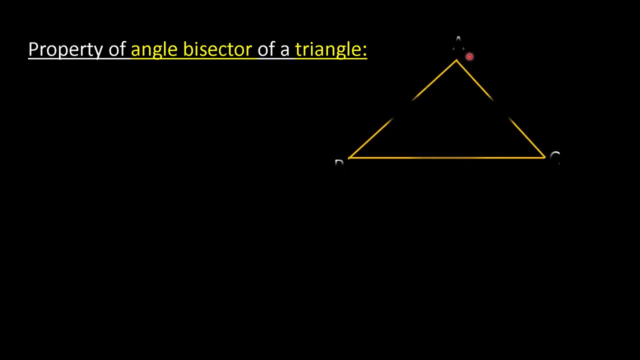 of concurrency is known as in center and it is denoted by capital I. so this point is in Center I. before we start to prove results, do we must first: this point is in center I. before we start to prove results, do we must first? let us understand the property of angle bisector of a triangle. let us 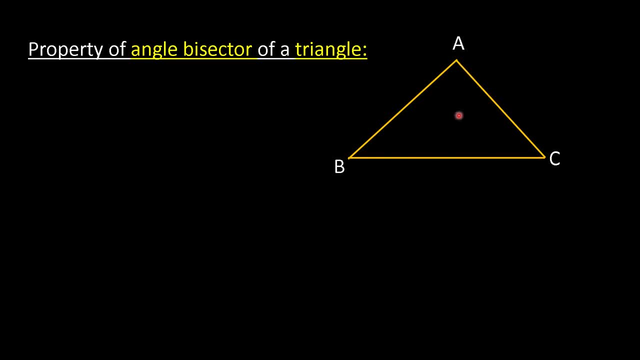 understand the property of angle bisector of a triangle. so we have triangle ABC here. side opposite to angle is BC. let side opposite to angle A be X, side opposite to angle E be Y and side opposite to angle C be Z. The property says that angle bisector cuts the side opposite to the angle. 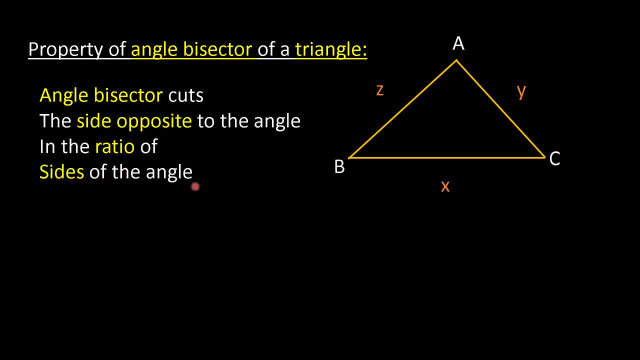 in the ratio of the sides of the angle, which means angle bisector AD of angle BAC cuts side BC, which is opposite to angle A. in the ratio Z as to Y, where Z is the side angle AB, Y is side AC. Angle bisector BE cuts side CA, which is opposite to angle B in the ratio. 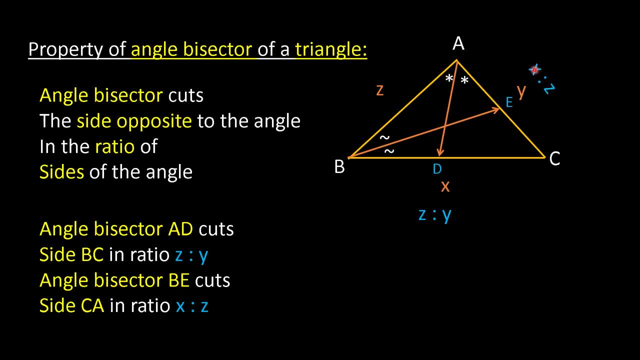 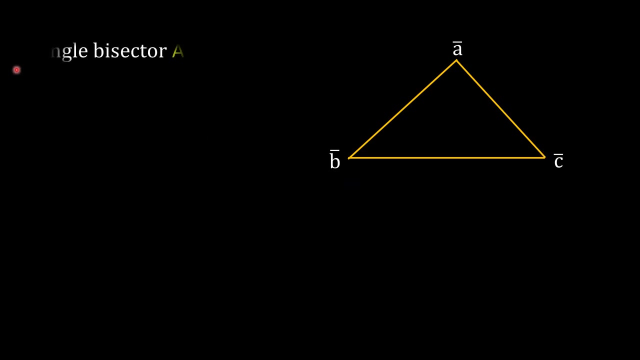 X as to Z, where X is side BC, Z is side BA. Angle bisector CF cuts side AB, which is opposite to angle C, in the ratio Y as to X, where Y is length AC and X is length BC. We have triangle ABC For angle bisector AD D cuts side BC in the ratio Z as to Y. 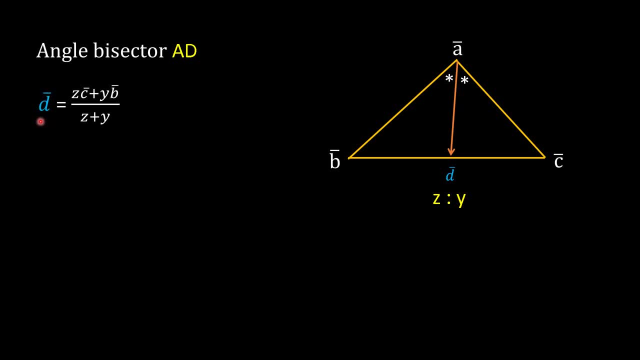 therefore, position vector D bar will be D bar equals ZC bar plus YB bar upon Z plus Y. Point E divides CA in the ratio X as to Z. therefore, position vector E bar will be E bar equals XA bar plus ZC bar upon X plus Z. And for angle bisector CF F divides side. AB in the ratio X as to Z And for angle bisector: CF F divides side AB in the ratio Z as to Z, And for angle bisector: CF F divides side AB in the ratio Z as to Z, And for angle bisector. 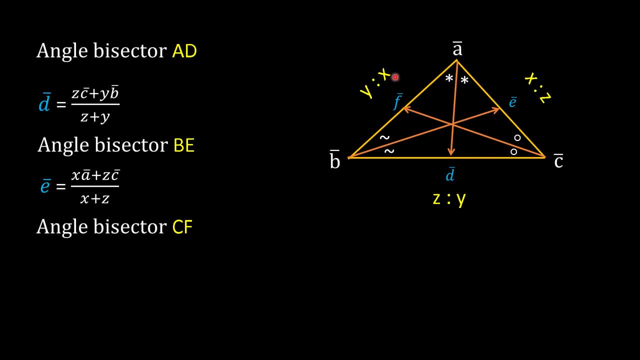 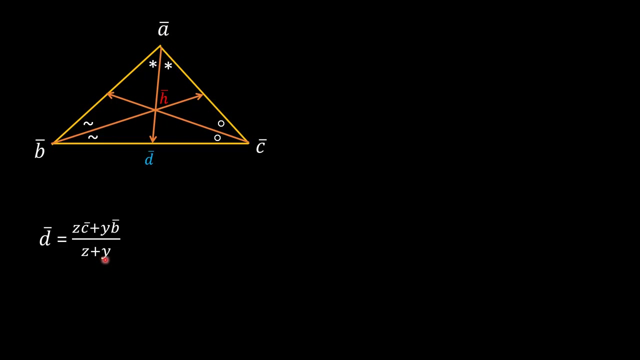 CF width dashboard and width is gonna be тебя bar y as to x. therefore position vector: F bar will be f bar equals yb bar plus xA bar upon y plus x. We have D bar equals ZC bar plus yB bar upon Z plus Y. 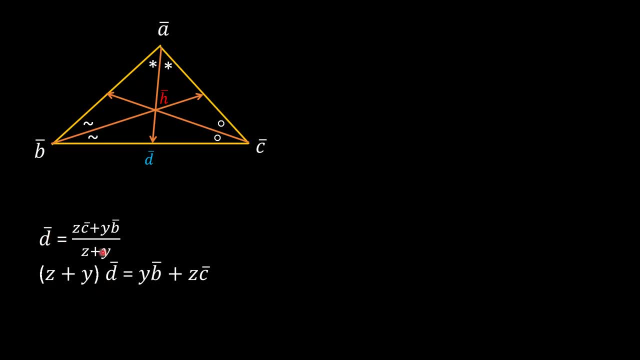 We will write Z plus Y as to Z plus X And for angle bisector À matrix, Seungnając Y s to Y, Y s plus X As to Y as to Z cIn each side we make the into D bar equals Y B bar plus Z C bar. there is X a bar lacking on the right. 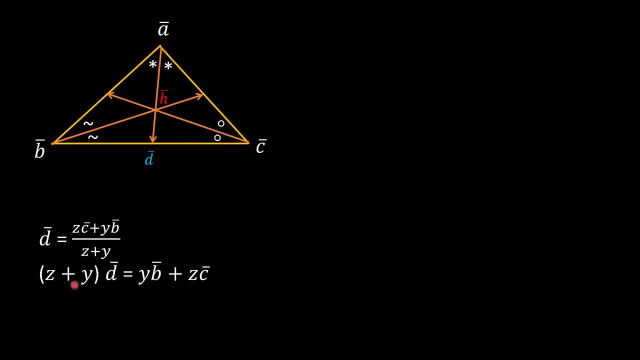 hand side. so we will add X a bar on both left hand side and right hand side. so it will be plus X a bar on the left hand side and X a bar on the right hand side. we will divide both sides by X plus Y plus Z. here the right hand side, X a bar. 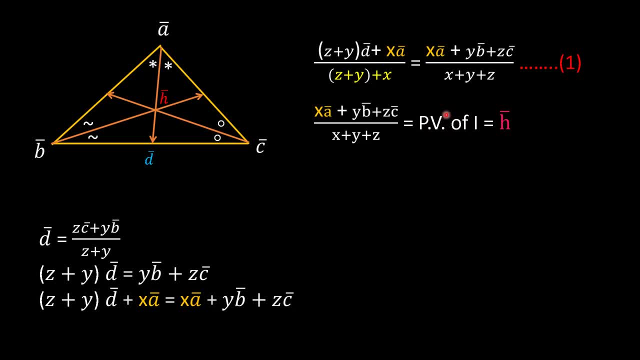 plus Y B bar plus Z C bar upon X plus Y plus Z is the position vector of the in-center eye, which is this point, and we denote it by H bar. therefore, we write: H bar equals Z plus Y D bar plus X a bar divided by Z plus Y. 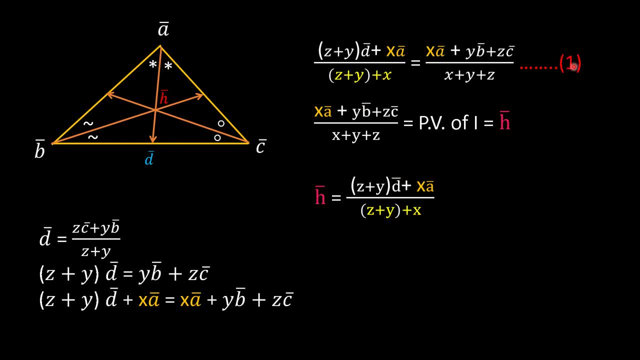 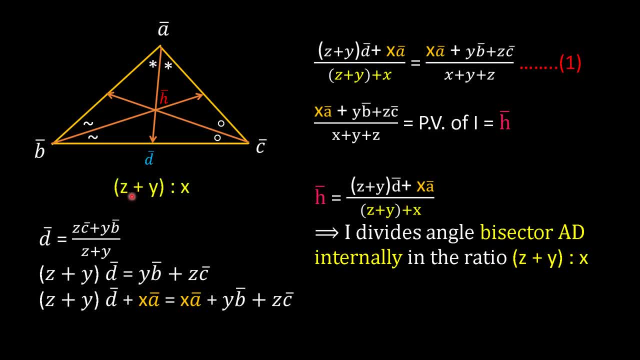 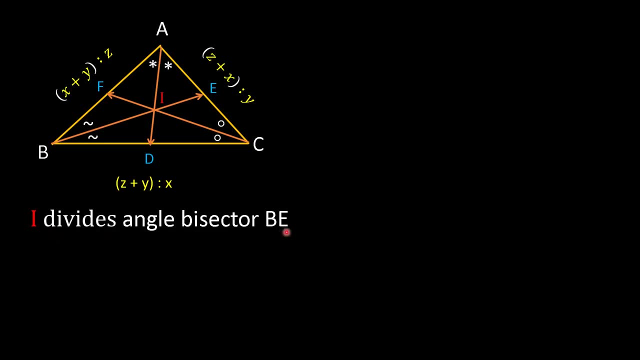 ad. internally in the ratio Z plus ad. internally in the ratio Z plus Y as to X, Z plus Y as to X. on the similar Y as to X on the similar Y as to X. on the similar lines. we can prove that I divides angle by sector PE. 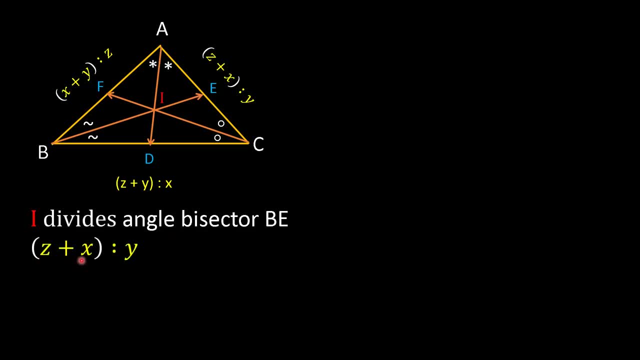 lines. we can prove that I divides angle by sector PE lines. we can prove that I divides angle by sector PE in the ratio Z plus X as to Y, in the ratio Z plus X as to Y, and I divides angle by sector CF in the ratio X plus Y as to Z. 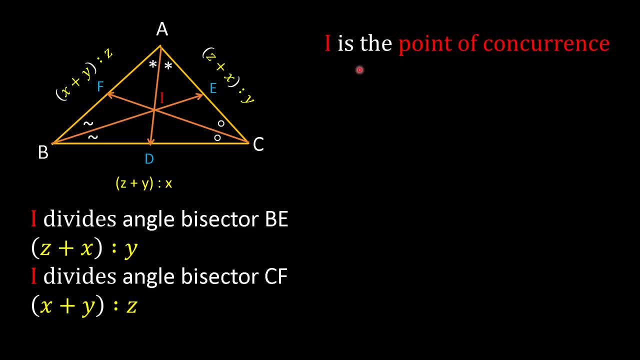 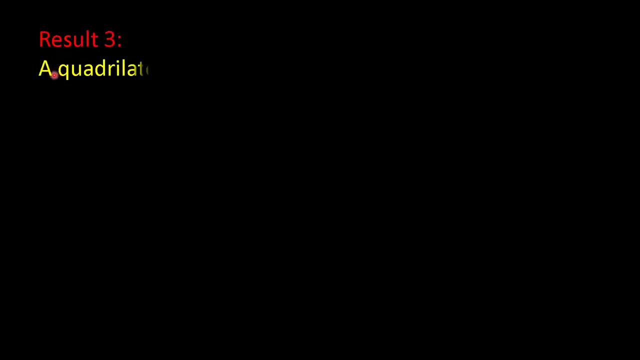 therefore, I is the point of, therefore, I is the point of concurrence of angle bisectors AD, PE and CF of triangle ABC. Chapter 4 says that a quadrilateral ABCD is a parallelogram if, and only if, its diagonals AC and BD bisect each other. 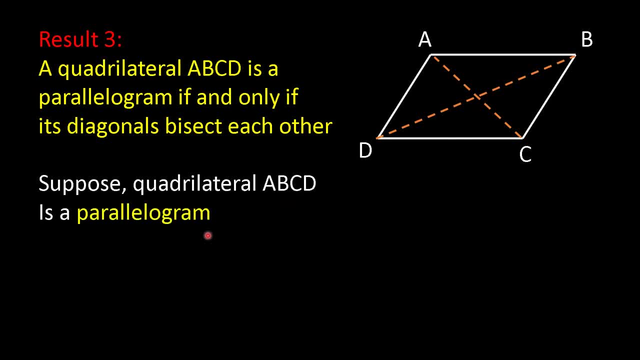 Suppose quadrilateral ABCD is a parallelogram. Therefore we have b bar equals dc bar, which we can write as b bar minus a bar equals c bar minus d bar. By rearranging the terms we will write it as b bar plus d bar equals c bar plus a bar. 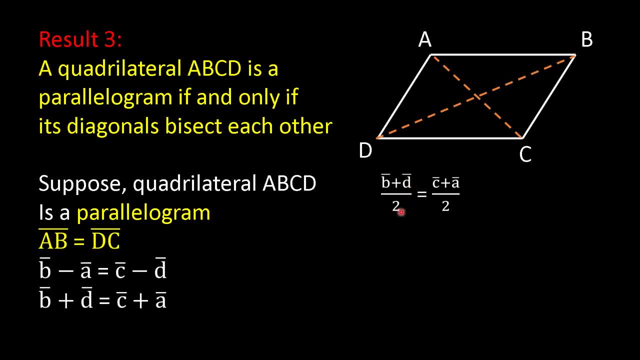 which will be b bar plus d bar by 2, equals c bar plus a bar by 2. But b bar plus d bar by 2 is nothing but the position vector of the midpoint of the diagonal BD, which is point E, and its position vector is E bar. 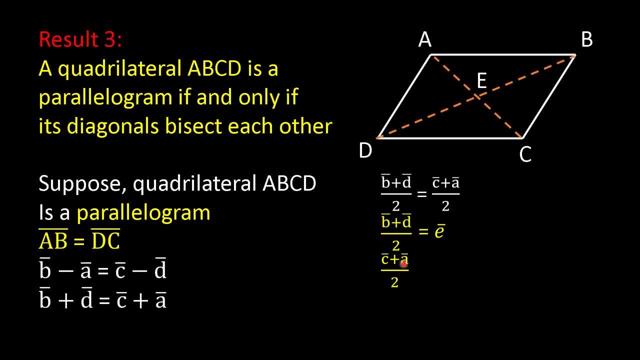 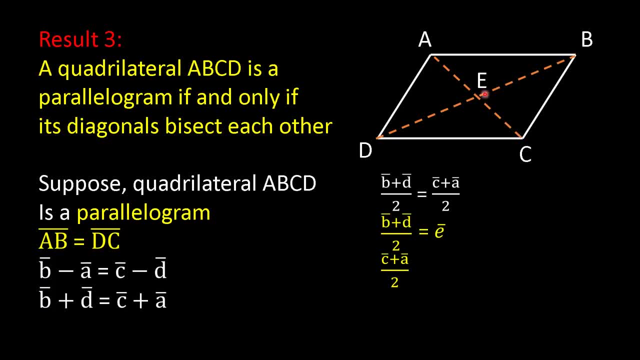 Similarly, c bar plus a bar by 2 is the position vector of the diagonal AC, which is E, and its position vector will also be E bar, Since the position vector of the midpoint of diagonal P, D and A C are one and the same, which is E. therefore, we can say that diagonals A, C and BD. 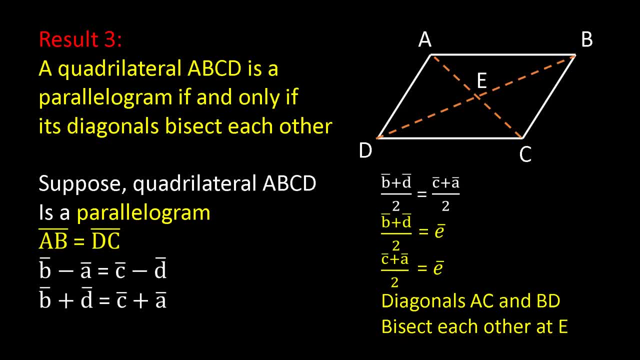 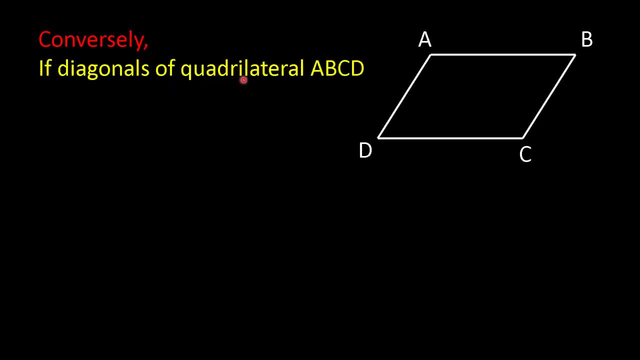 Bisect each other. at E. We can prove its converse also, which says that if diagonals of a quadrilateral ABCD bisect each other, then it is a parallel cramp, Since diagonals AC and BD bisect each other. therefore we can write: 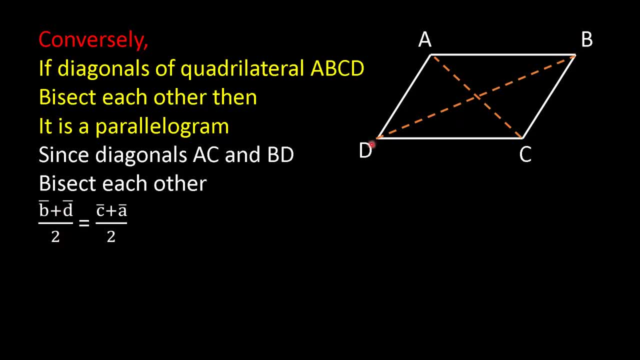 b-bar plus d-bar by 2 equals c-bar plus a-bar by 2, which will be b-bar plus d-bar equals c-bar plus a-bar. We will rearrange the terms and write: b-bar minus a-bar equals c-bar minus d-bar. 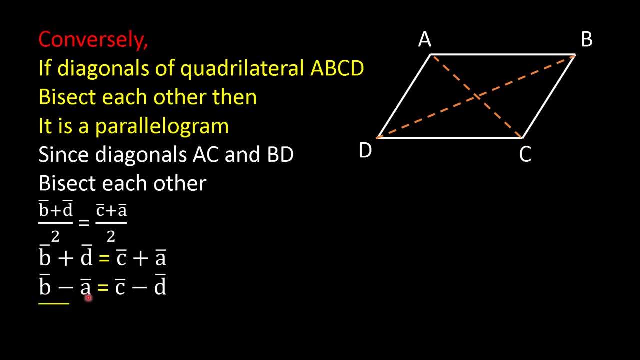 Now b-bar minus a-bar is a parallel cramp. Since b-bar is nothing but ab-bar and c-bar minus d-bar is dc-bar, we can say that side AB is parallel side DC and side AB equals side DC, which proves that ABCD is a parallel. 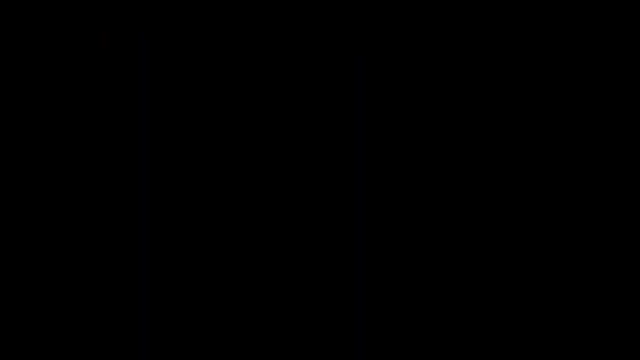 cramp. We will prove result 4, which says that the median of a trapezium- this is trapezium ABCD- EF is the median. it is parallel to the parallel sides of the trapezium. Median EF is parallel to parallel sides AB and DC. 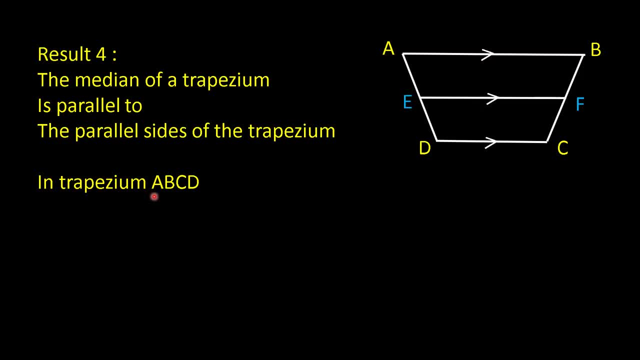 In trapezium ABCD, AB is parallel to DC. therefore, it is sufficient to prove that EF-bar is parallel to DC-bar. Since AB-bar is parallel to DC-bar, we write: AB-bar equals a non-zero scalar root of a non-zero. 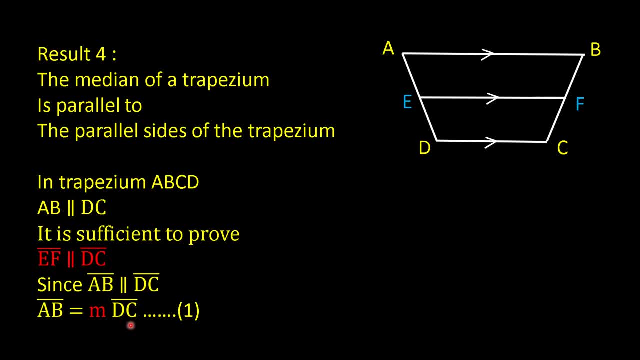 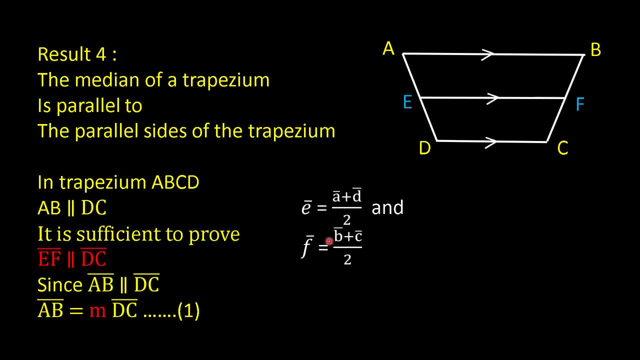 midpoint of BC we write: F-bar equals b-bar plus c-bar by 2.. So EF-bar will be F-bar minus E bar. F bar is B bar plus C bar by 2.. E bar is A bar plus D bar by 2.. By rearranging 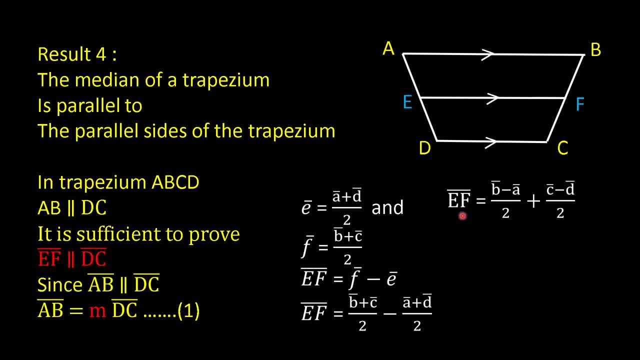 the terms we will write: E F bar equals B bar minus A bar by 2, plus C bar minus D bar by 2.. But B bar minus A bar is AB bar and C bar minus D bar is DC bar. Therefore E F bar will be AB bar by 2 plus DC bar by 2.. We name this equation 2.. But from equation 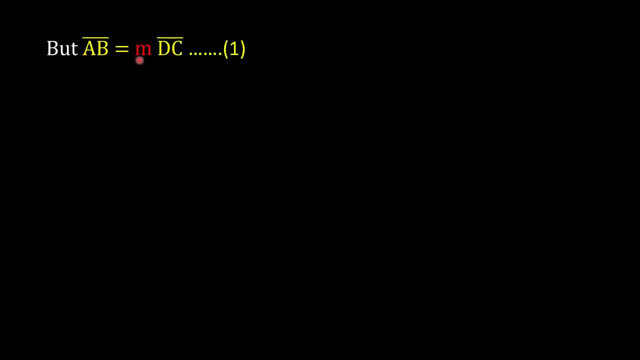 1, we have AB bar equals M times DC bar. So E F bar will be MDC bar. putting MDC bar in place of AB bar by 2 plus DC bar by 2, which will be M plus 1 by 2 times DC bar, which will mean E F bar is parallel to DC bar. So 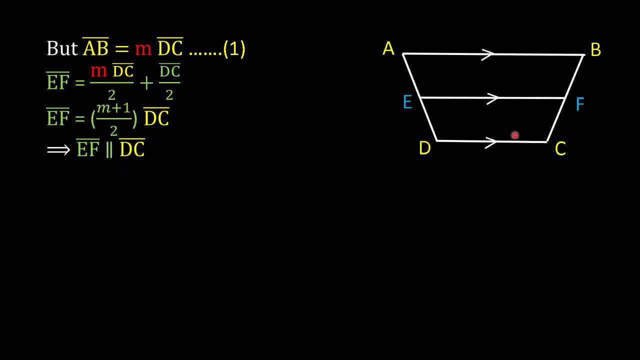 this is trapezium, ABCD and medium, Which means that E F bar equals RDB. The second equation will be, of course, problem B, when E F bar is parallel to RDC bar. Therefore E F bar equals MAC ratio. equal. 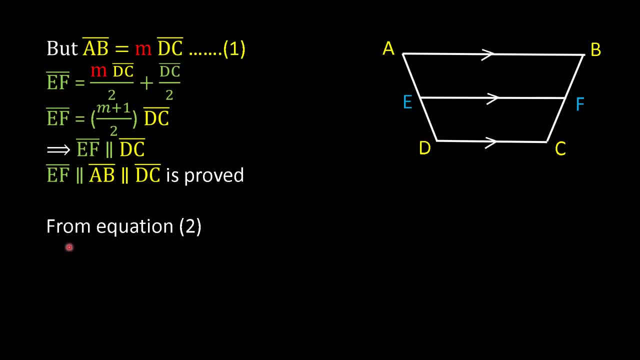 to DC bar by 2.. So this equation 1 gets E F bar equals the standard position of E F bar is parallel to side DC bar. Therefore we can say that E F bar is parallel to AB bar is parallel to DC bar is proved. Now from equation 2 we have: E F bar equals AB bar by 2 plus DC bar by 2, which we can��요as. therefore we can say that E F bar equals AB bar by 2 plus DC bar by 2, which will be, if you write. 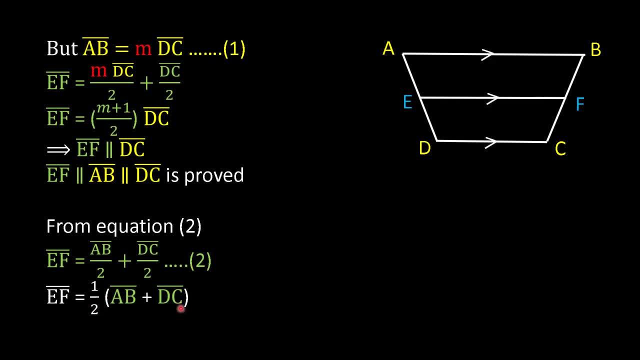 half times AB bar plus DC bar. but since AB bar is parallel to DC bar, we can directly add their magnitudes. therefore we write: EF equals half times AB plus DC, which is the length of median is half times sum of the lengths of the parallel sides. this statement is proved. 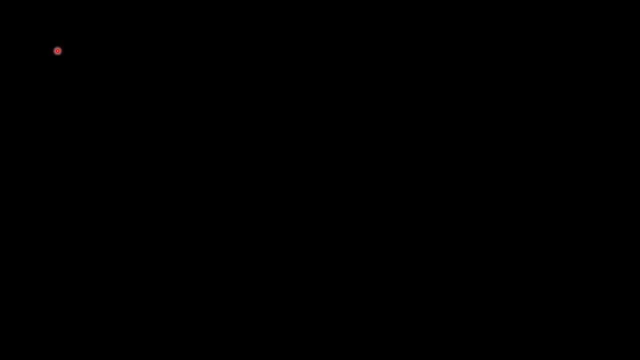 in result 5. we have to prove that angle subtended on a semicircle is a right angle. draw a circle, so this will be semicircle with radius R and center at the origin. center at the origin AB is diameter and C is any point. 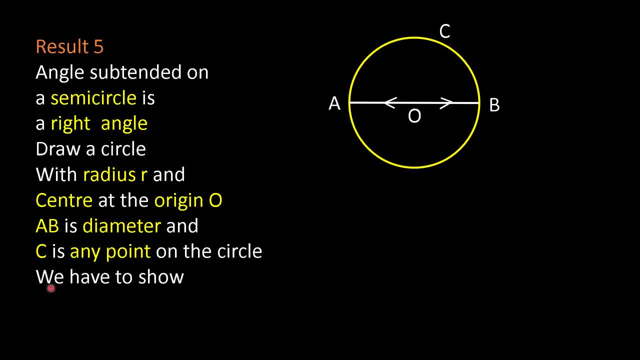 on the circle. we have to show that angle ABC equals 90 degrees. angle ABC is 90 degrees. since O is origin, mod C bar equals 90 degrees. since O is origin, mod C bar equals 90 degrees. since O is origin, mod C bar will be R. also, mod A bar will be equal to mod B bar will be equal to R each and B. 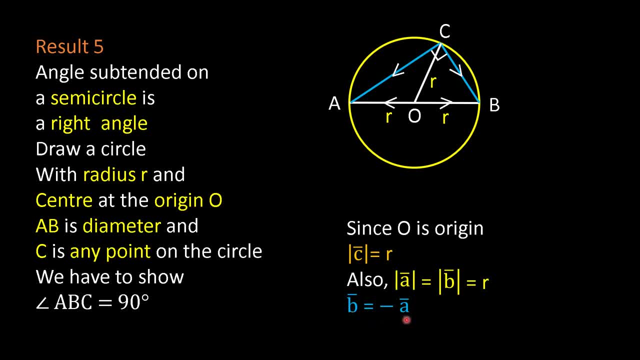 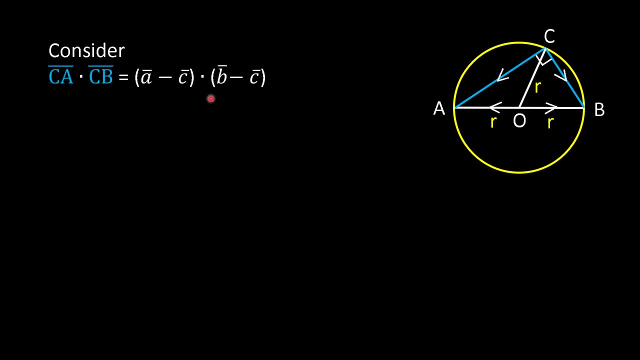 bar equals minus A bar, because B bar and A bar are oppositely directed from the figure. consider CA bar dot CB bar, which will be A bar minus C bar. dot B bar minus C bar, but B bar is minus A bar. therefore, in place of B bar, we will put minus A bar, it will be minus. 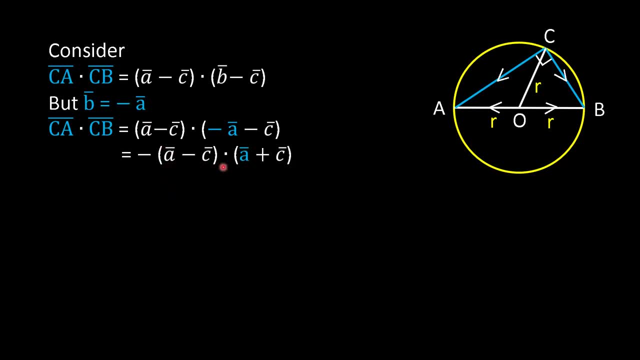 times A bar minus C bar. dot A bar plus C bar, which will be minus A squared, minus C squared, but A equals C equals R. therefore CA bar dot CB bar will be minus R squared, minus R squared, which will be 0. since CA bar dot CB bar is 0, we conclude that CA bar is perpendicular. 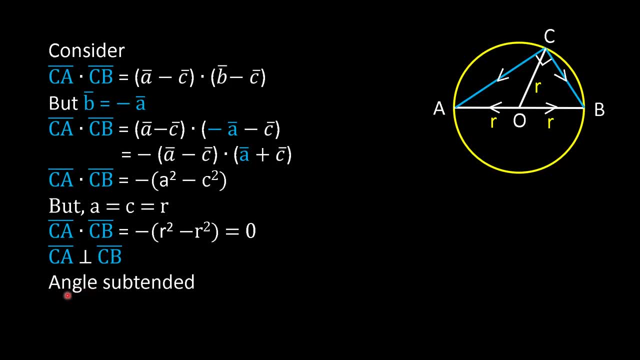 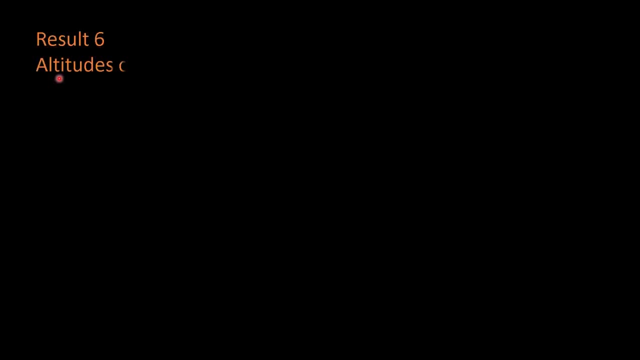 CB bar. therefore, angle subtended on a semicircle is a right angle and angle subtended at an angle equal to side, this angle is equal to nuevas umbershorizontal value. Let us go through the left side program. In result 6, we will show Altitudes of a triangle are concurrent In triangle. ABC, AlphaD, AlphaBở, 올�إnd was chosenadt and γзд. 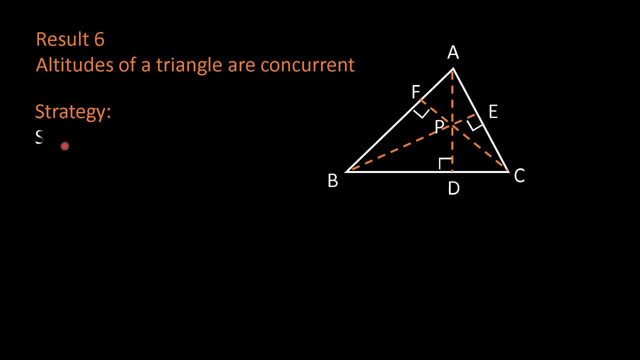 We will use the strategy that, since altitudes BE and CF intersect in point P, all we need to show is AP bar and AD bar are collinear, That we will start by showing. AD bar perpendicular BC bar In triangle ABC. BP bar is perpendicular AC. 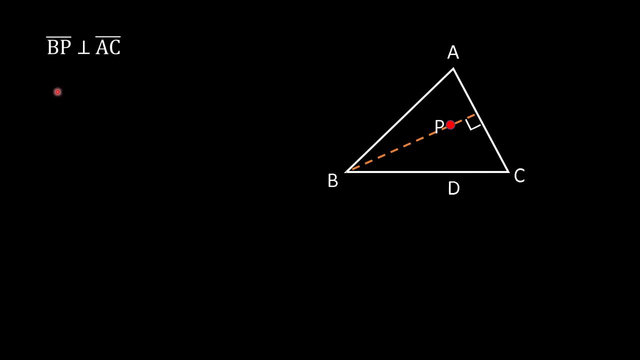 bar. Therefore dot product BP bar. AC bar will be zero. BP bar will be BC bar minus BB price. AC bar will be CBar minus A bar, Which will be BBar dot CBarr minus BBar dot A Barr minus BBar dot CBarr. 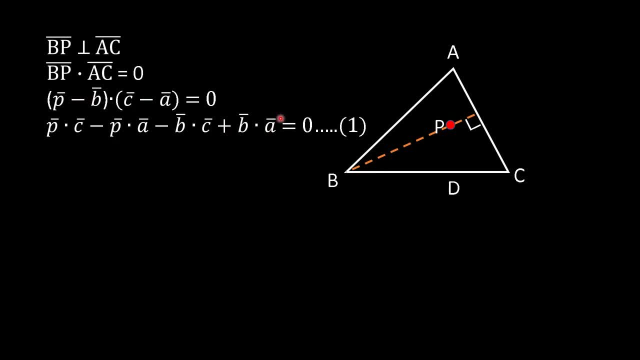 plus BBar dot A Barr plus BBar dot A Barr equals 0.. We name this equation 1.. Also, Cp bar is perpendicular to Ab bar. Therefore, Cp bar dot Ab bar will be 0.. Cp bar will be P bar. minus C bar, Ab bar will be P bar. 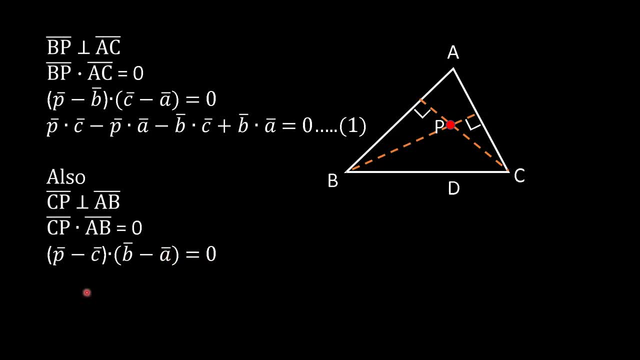 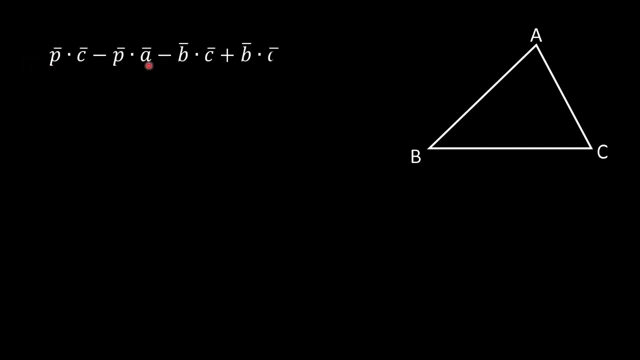 minus Abar equals 0. It will be P bar dot P bar minus P bar dot Abar minus C bar dot. P bar plus C bar dot Abar equals 0.. We name this equation 2.. We will rewrite these two equations and subtract equation number 2.. 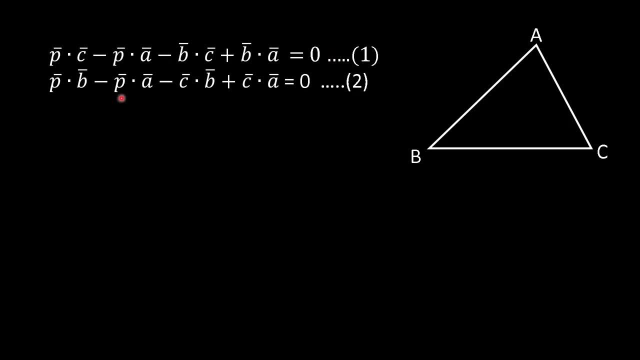 from equation number 1.. For that we will change the signs of the terms of equation number 2, So this plus becomes minus, minus becomes plus, minus becomes plus, and this plus becomes minus, And we get P bar, dot, C bar minus P bar. 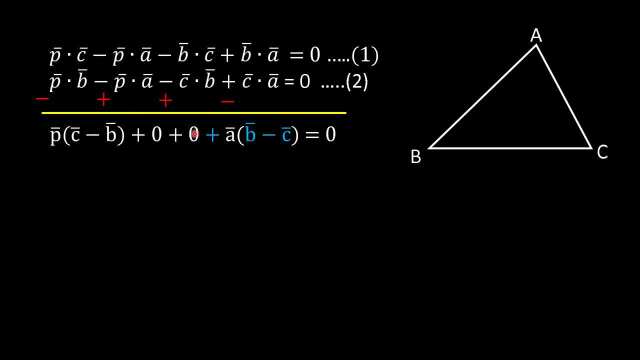 This is C bar minus C bar. dot C bar will be zero. this will be zero. this will be a bar times b bar minus c bar, which is zero. we will write this b bar minus c bar as c bar minus b bar and change this plus sign to minus sign. 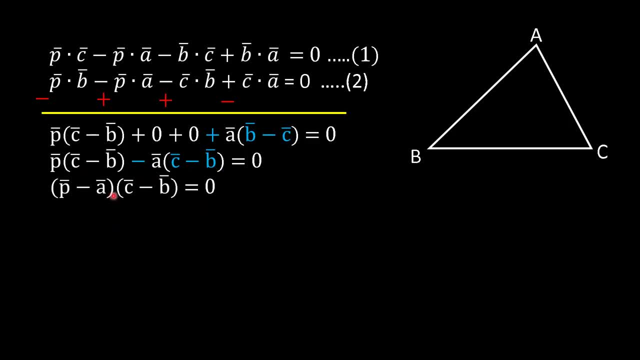 we will write this as: p bar minus a bar, multiplied by c bar minus b bar. p bar minus a bar will be a p bar and c bar minus b bar will be b c bar. so a p bar dot b c bar will be zero, which means that a p bar is perpendicular to b c bar.